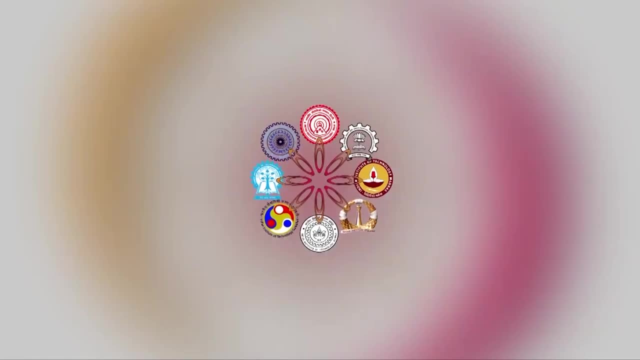 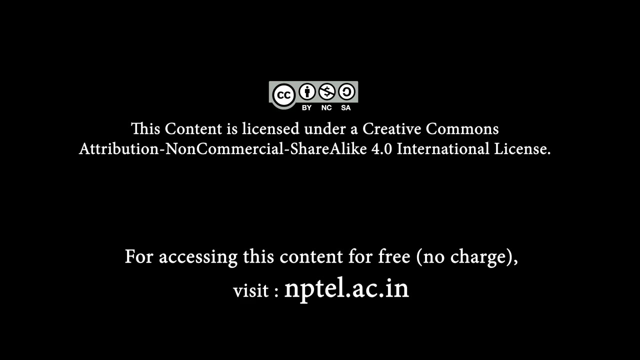 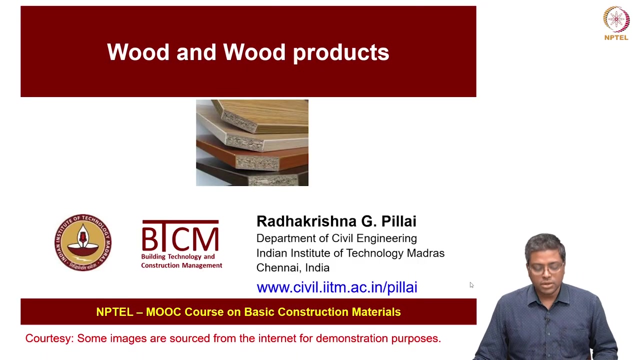 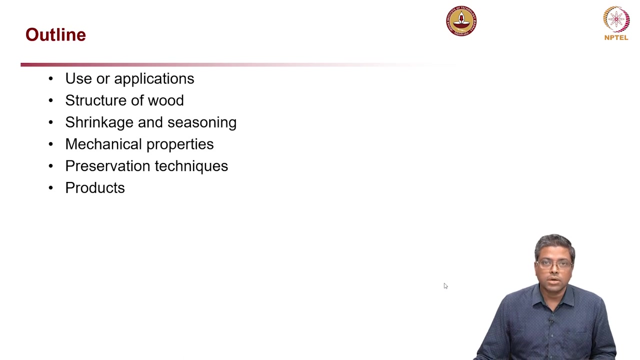 Hi, I am Radhakrishna Pillai from IIT Madras, As part of this MOOC course on basic construction materials. today, this lecture will cover wood and wood products and we will talk about use or applications of wood. and then we will look at the structure of the wood: how is it made? 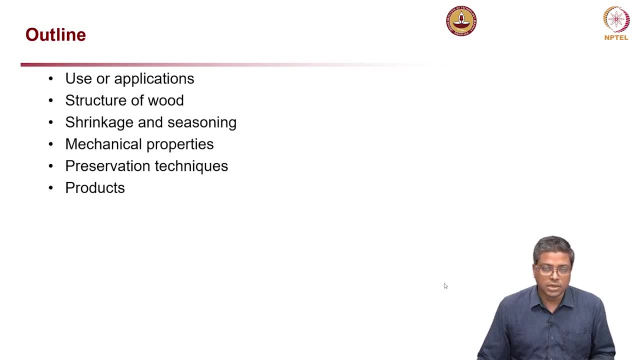 and then look at shrinkage and seasoning, like shrinkage related problem, and then how to address that- one of the method is by seasoning- and then look at the mechanical properties of wood and then also very briefly on preservation techniques and the and couple of products also, we will look at and then even when we talk about those products, how the damage mechanisms. 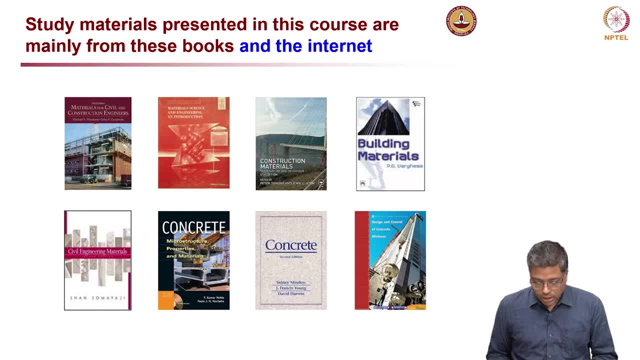 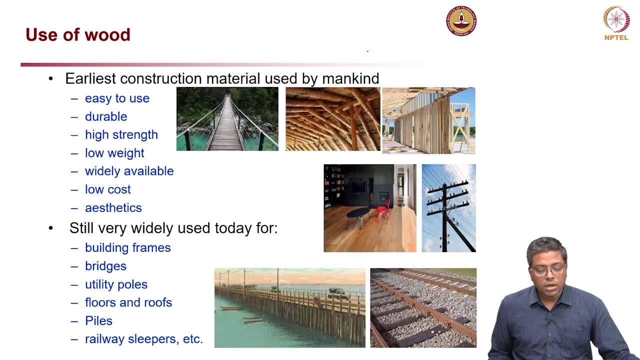 etc will also be discussed. As I have been telling, this course is made, you know, with inputs from various textbooks, as we see here, and also lot of photographs etc from the internet. So the use of wood or the where we, where do we apply or use this? you know, use wood. 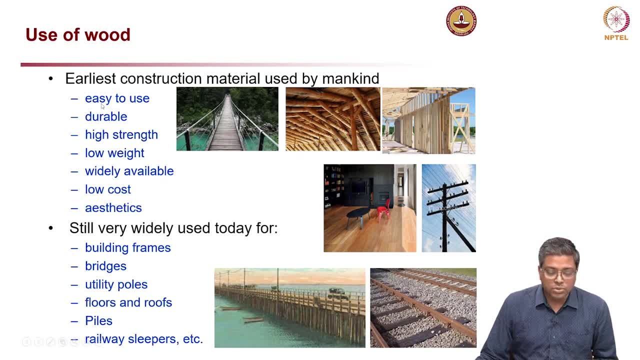 So it is one of the earliest construction material used by the Manken and why we were using it? because it is easy to use and it is durable and it is having high strength. I mean, depending on which direction you are using and what you are using it for, or what. 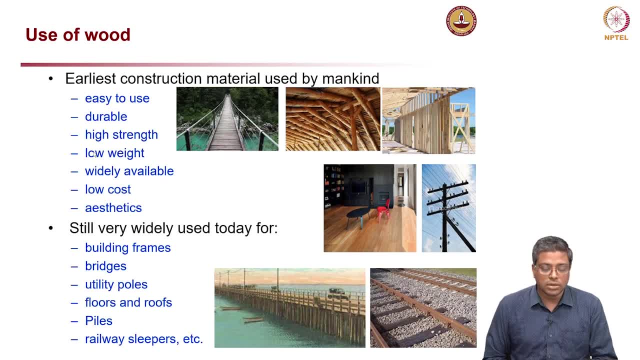 type of load is applied, in which direction it is applied- all that we will discuss in detail. So these are the coming slides. and also it is a light weight. So we talked about easy to use, durable, high strength, low weight and widely available. okay, low cost and it. 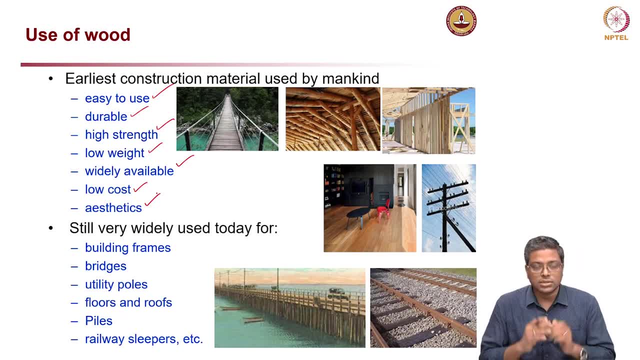 also looks good because of the grains and the structure, which is, I mean, the design, you know grain structure and all that gives you good look also and relatively low cost compared. I mean depends, I mean there are some additional requirements for the sleepers, but it has been used widely. 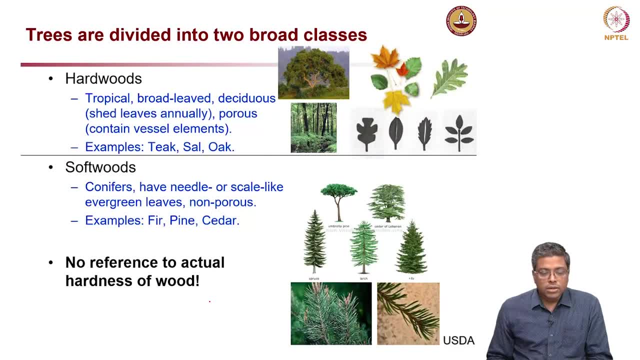 in the earlier time. okay, Now, trees in general can be divided into two broad classes. one is hardwood and the other one is softwood. okay, So this- I am just put this for some information purpose, I mean, so you can see, hardwood is. 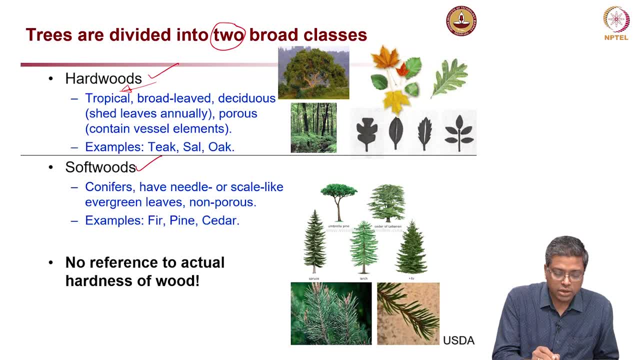 generally available in tropical climate conditions conditions- okay, tropical climate conditions. Generally the leaf structure. you can see the top half of the screen and bottom half of the screen. there is a strikingly different structure or the visual, I mean the appearance. 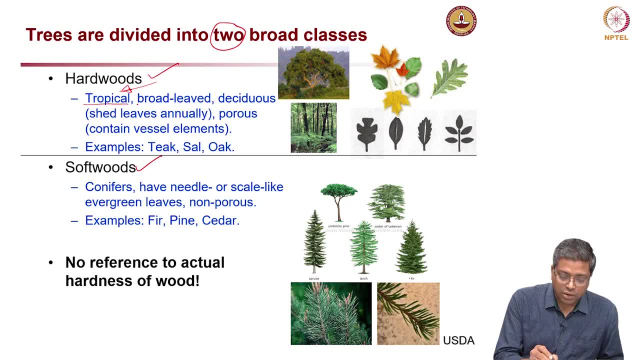 is very different of the leaves. So in the case of hardwood it is broad-leaved and deciduous. that means they shed leaves annually, okay, And they are generally porous in structure and examples are teak, sal, oak, etc. that. 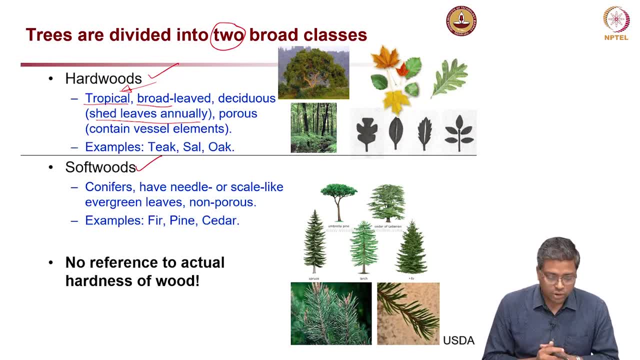 comes under the classic class of or category of hardwood. Then we have softwood, which are conifers and have needle or scale like evergreen leaves- okay, non-deciduous and then non-porous also. examples are fir, pine, cedar, etc. 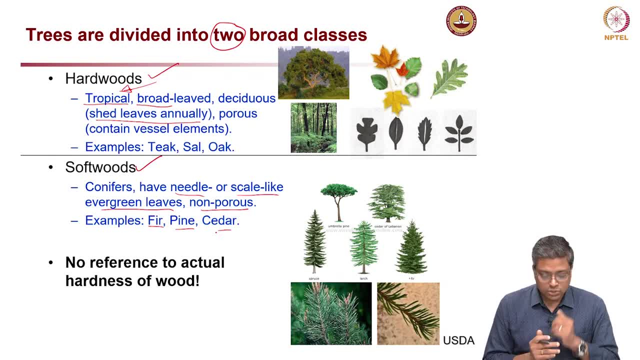 But now just these two classifications. You can look at what type of geographical location or climatic condition these two types of woods are present. Now, one more important thing is this name: hardwood and softwood does not reflect on the mechanical hardness of the wood. okay, 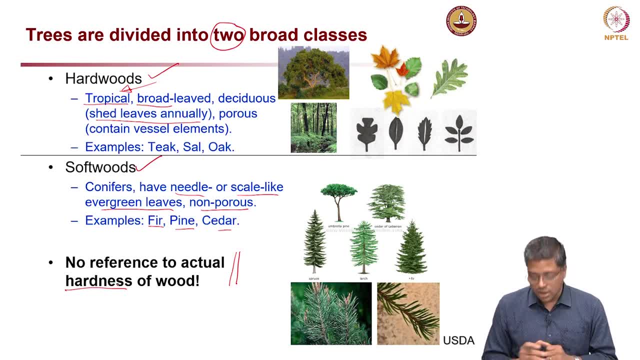 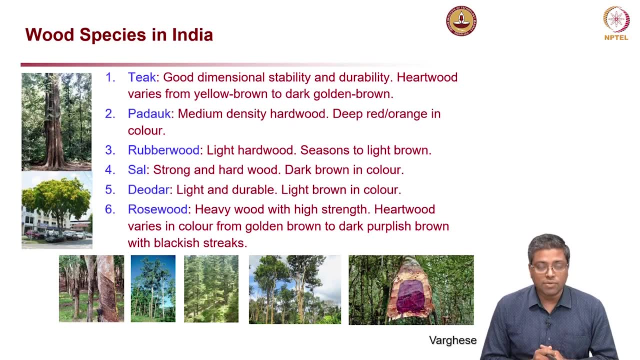 This hardness of the wood has nothing to do with these terminologies of hardwood and softwood. okay, just remember that. Then, what are the type of wood or species available? in India, We generally use teak a lot because- mainly because- it is easy to work with. 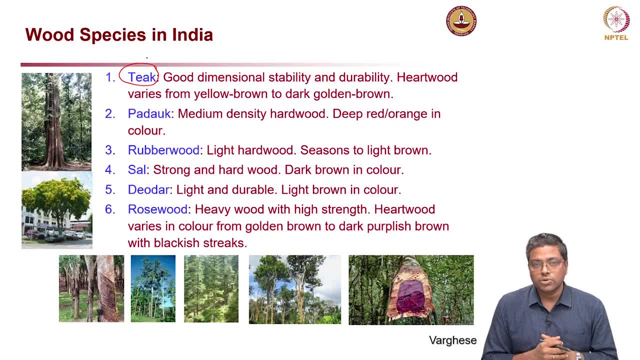 If you ask a carpenter- you know what is the advantage of using teak wood. they will say it is easy to work. In other words, you do not need much energy to you know chisel or to work with that. 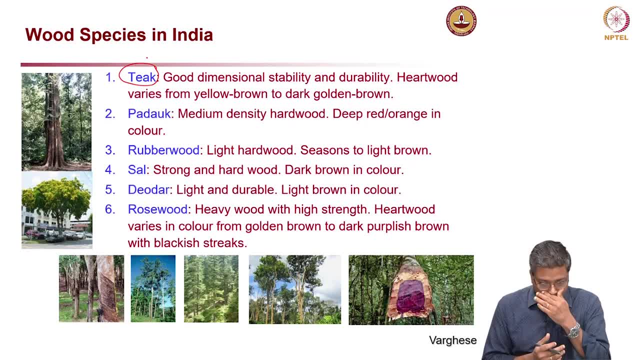 to cut that wood, to work with that wood. okay, it is easy to work with. that is if you ask the carpenter. okay. So also another technical reasons are it has good dimensional stability. That means it does not shrink or swell, you know, as a function of time. I mean it does. 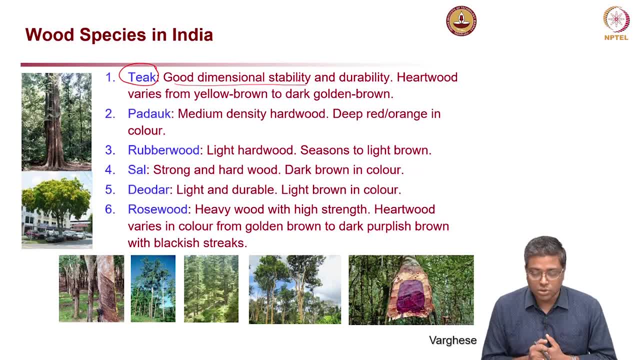 not shrink or swell as much as other type of wood and it is durable. That is why it is very, very costly also. Then density also matters. So padak is another type where it is medium density. hardwood color also matter. So you can look at this list here. 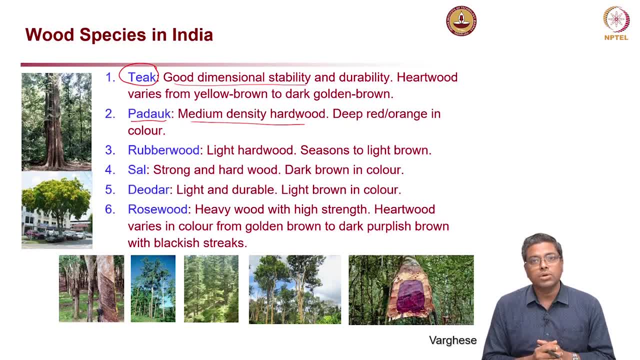 I mean, this is not something to memorize- is just for you To have a feel of what type of timber or wood are available in our country then, and what are the properties you should look for. also, Color is definitely one thing, because aesthetics is a function which we look for. 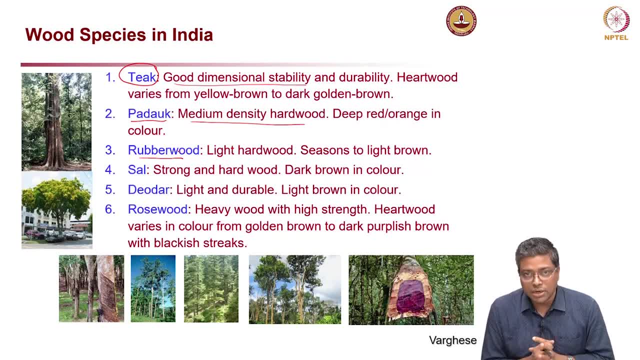 And also the dimensional stability, strength, how easy it is to work with the timber, the wood. these things we should really worry about. I have been using this word- timber and wood Wood in between. If you really look at definition for this, timber is nothing but a processed wood okay. 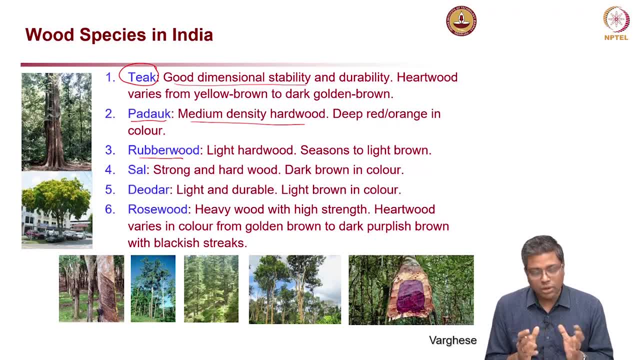 But more or less. I do not think it really matters. You can kind of use both words. But timber in general, when we say it is a processed wood, okay. Now other types are sal, deodorant and rosewood. These are all available in various parts of our country. okay, 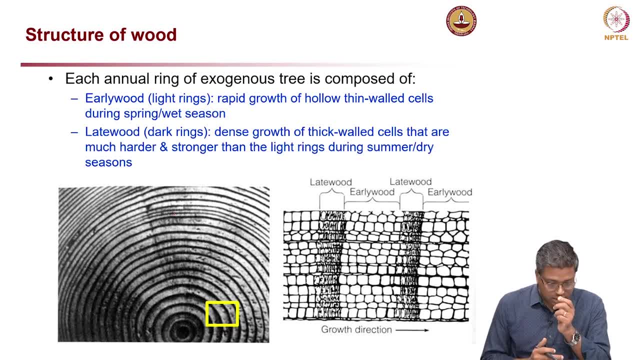 And now let us look at the structure of wood. So each annual you can see the picture on the bottom left. This is the typical cross section. If you take, if you cut a tree, you will see it like rings like this. okay, 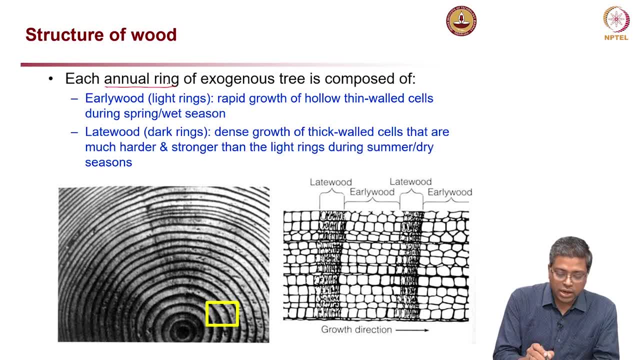 Now, these are like. each ring represent one year, okay, each ring in this. So by looking at this cross section of the wood, we can tell the age of that wood, okay, or age of that tree, We can tell. Now look carefully on the picture. 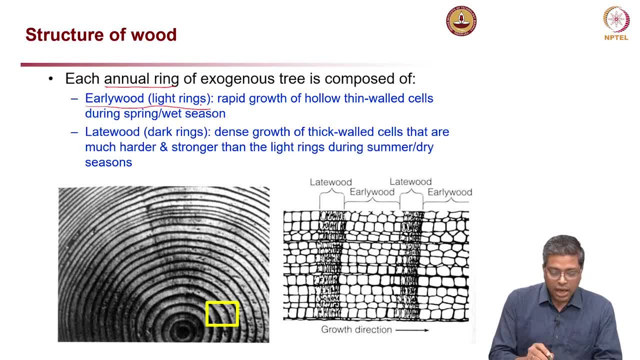 You can see an early wood which are light rings and a late wood which are dark rings. Now on the right side, bottom right side- you have a close-up image of this yellow region which are shown in the left side image. It is a close-up view. 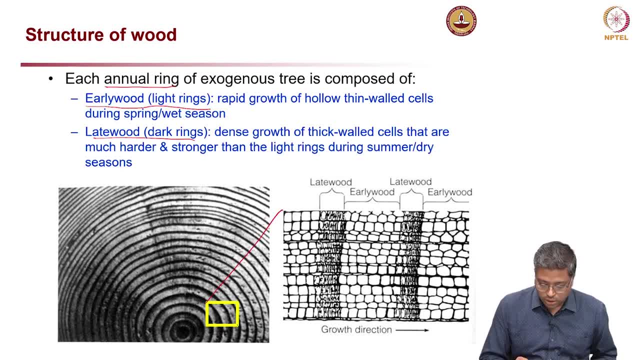 On the right side you have a close-up view. So this is something like this. okay, So this is the close-up view of this yellow region. Now look at this dark and you know light color and the dark color rings. 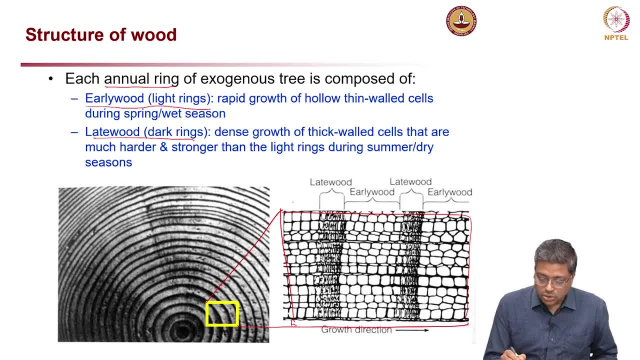 It is very clearly shown on the right side image. So this region- you can see early wood here. These are the light color region and the late wood, which are the dark color region. okay, So you can see that late wood is more dense, like this region is more dense and early wood. 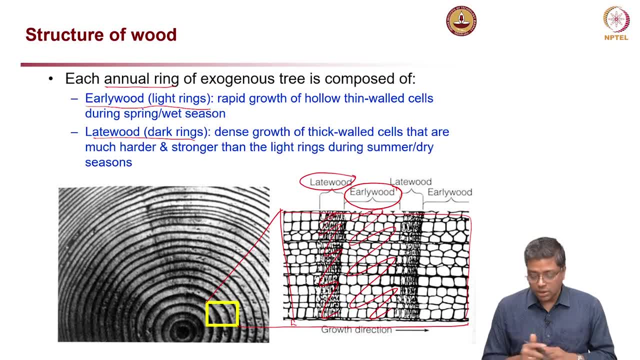 is less dense. This region is less dense. Okay, So that is clear. So two types of in the same in the when you form the ring. So what now? look at why this late wood and early wood. okay, 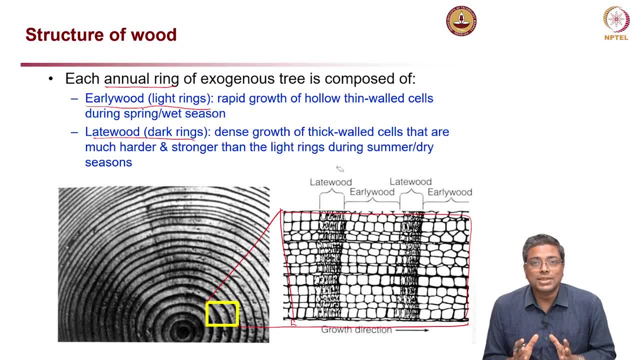 Now early wood. it is like a rapid growth of hollow, thin walled cells. This is the early wood we are talking. okay, You can see, in this region you have larger cell walls. They are hollow and they grow rapidly. Okay, 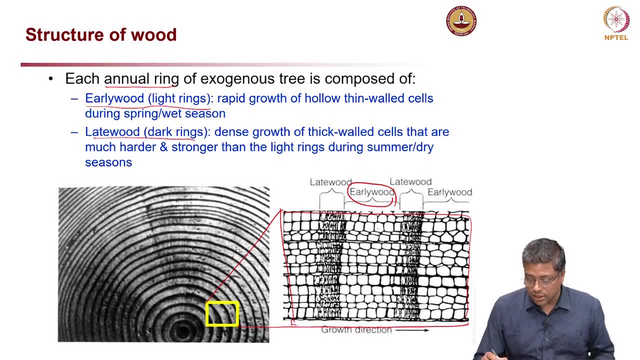 During the spring or wet season. that is when they grow rapidly, because whichever cavities are formed that will get filled with this moisture. So they kind of have a. eventually they will have a larger cavities, okay, or the cell structure is like that. 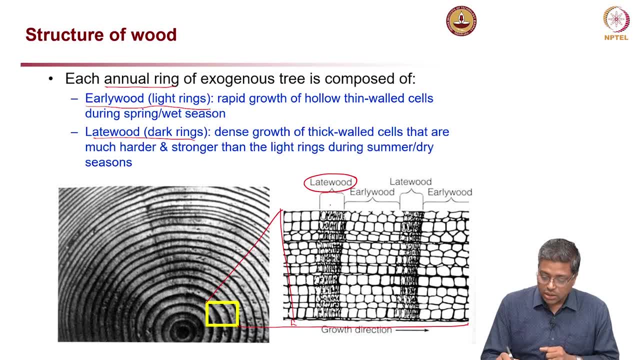 Now, when you talk about the late wood, which is this, you can think here, this denser region, and these are thick walled cells. Okay, So early wood, they are thin walled cells. Now, these late wood are formed during the summer or dry season, and they are thick walled. 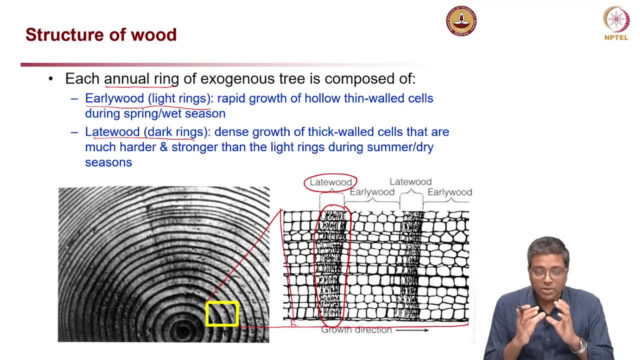 cells and smaller in size also. The cavities are also smaller and hence, because they are thick walled, they are much harder and stronger than the light rings. Okay, So this is the main thing to learn about these different rings and the region of the ring. 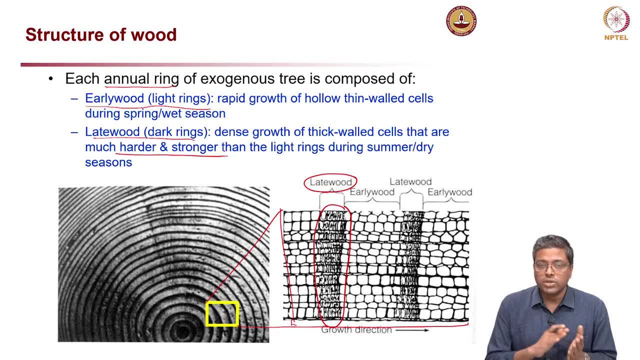 Late wood and early wood. Okay, Which one is stronger, which one is weaker in comparison, and which is formed in which time of the year? Okay, And then the reason for the. you know the strength, because you have thick wall, the. 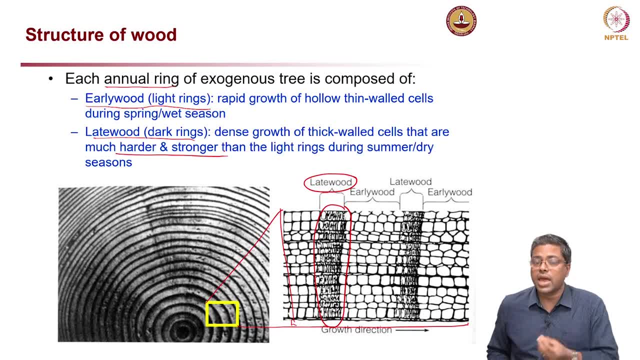 wall thickness plays a major role and the size of the cavities also plays a major role. If I look at here, this is the cavity. I am talking, I am drawing on the picture here. This is the cavity and this is the wall thickness. 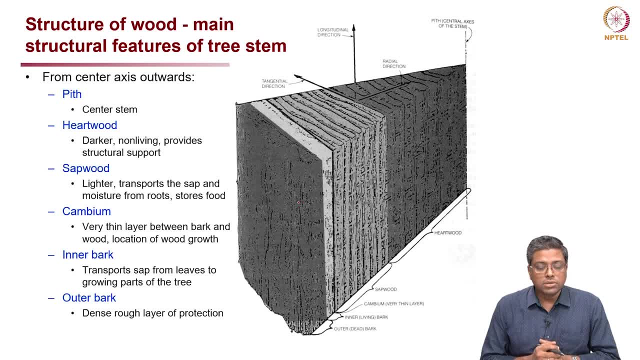 This is the wall thickness which I am talking, or the wall Now. structure of the wood, main structural features of a tree. if you cut a tree, Okay, These are all the different parts of a stem. Okay, You can see here. the first one is the central axis of the stem. 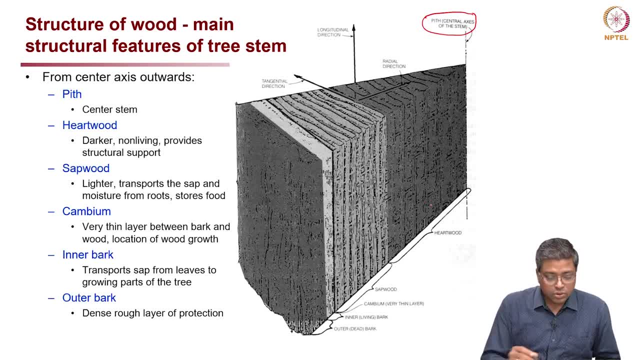 Okay, We call it pith, and then you have something called hardwood. that is here. I am just connecting the image and the text. Okay, So hardwood is the core of the wood, is darker and we say it is non-living and it provides. 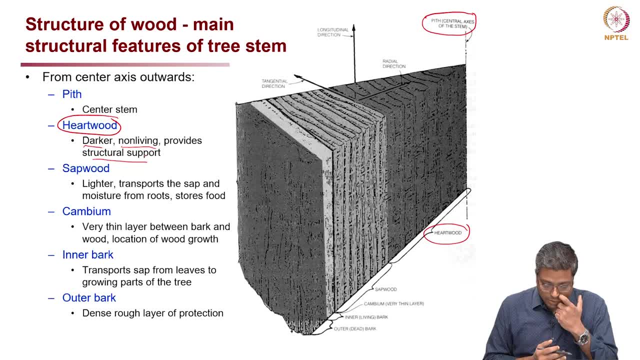 a structural support. Okay, It is not actively growing or it is a structural, provides a structural support. Then you have sapwood, which is the lighter color region here, and it transports the sap and moisture from the root and stores the food. Okay, 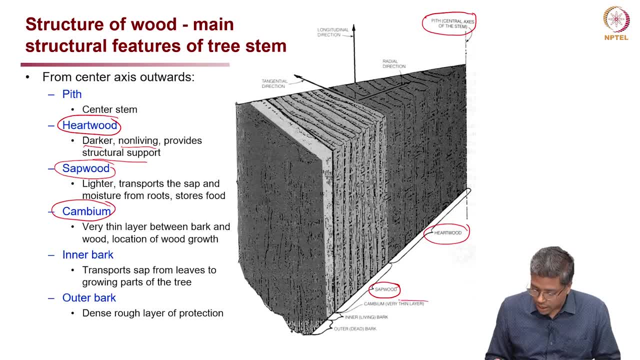 Then you have cambium. Okay, This is the outer and outer. You have cambium here, which is a thin layer, Okay, So you can see here, just thin layer is what we are talking. This thin layer, darker color region, you can see there. 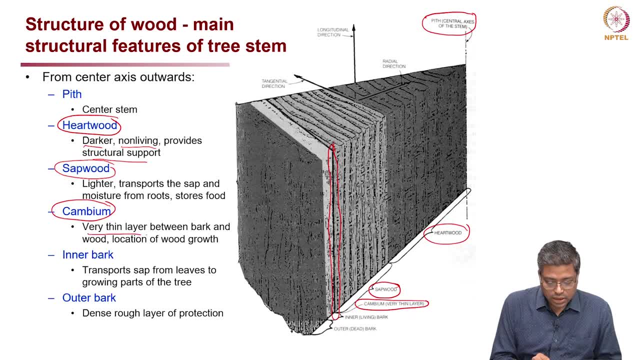 That is the cambium. And what is it? It is a very thin layer between the bark and the wood. Okay, Location of wood growth, That is where the wood grows laterally. Cambium- Now inner bark is another Bark- is kind of a thin layer. 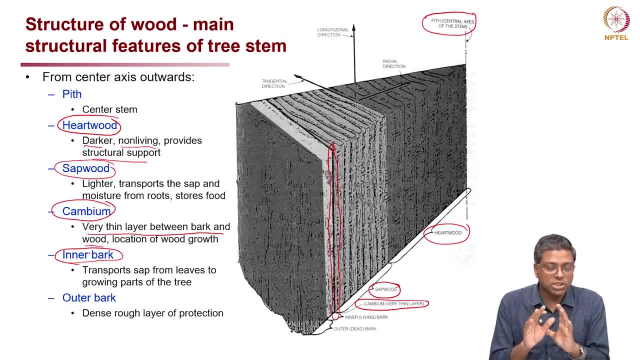 Okay, This is the outer and outer. It is kind of looked at as the outer shell of the core wood and the inner bark and outer bark. There are two categories for this. I mean two regions for this bark. So inner bark: transport the sap from leaves to the growing part of the tree. 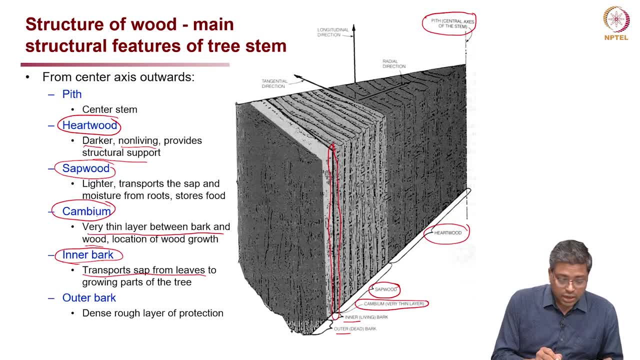 Okay Now, which is that growing part of the tree? That is the cambium. We just discussed that. Now, outer bark is the dense or rough layer, just for protection. Okay, So this portion here, it is just for protection. So this is, in generally, what if you take a timber or if you cut a wood, you can look. 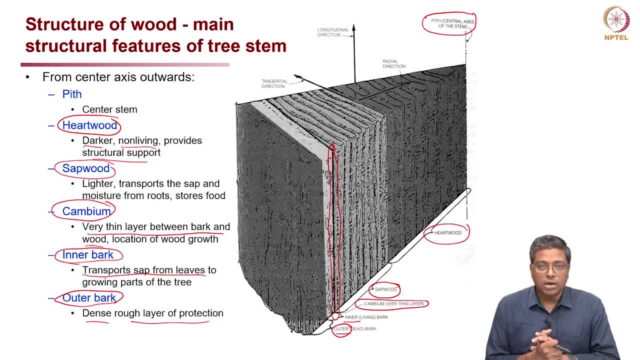 at the cross section and you can see these different regions, or you know, on a wood. Now there are also another important thing which we need to look at is the direction: Longitudinal direction, tangential direction and radial direction. I will discuss this. 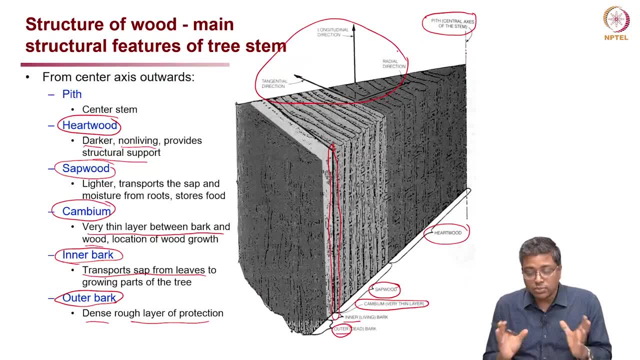 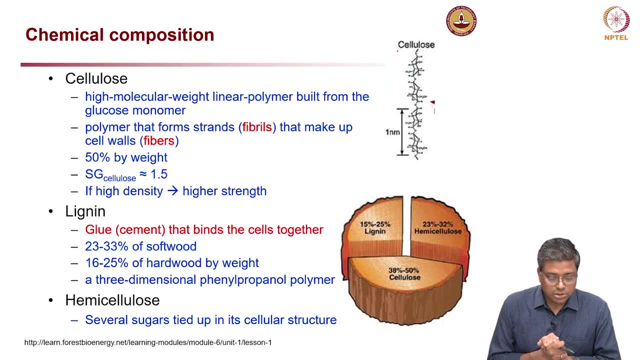 later. But remember that the properties change as we look at timber in different directions. Okay, Now chemical composition. What is the chemical composition In general? wood? you can look at the graph on the bottom right. there are three key components. 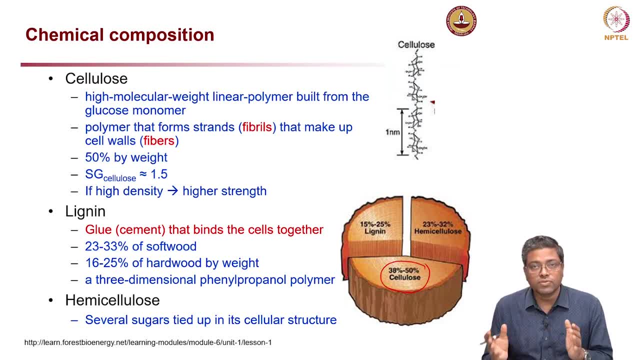 One is cellulose, which constitute about 40 to 50 percentage, and then you have hemicellulose, and then you have lignin. Okay, So the composition you can see. Cellulose is, You know, the major component, and then you have about 20 to 30 percent hemicellulose and 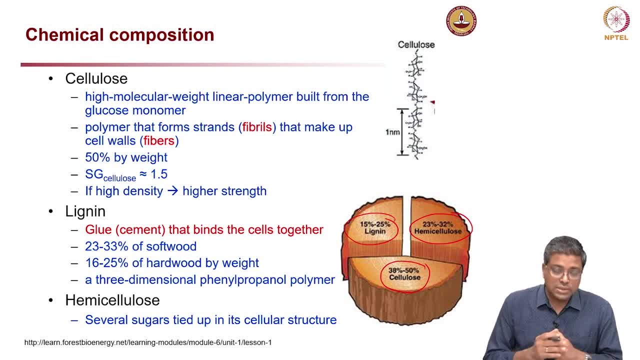 then 15 to 25 percent lignin. Now, what are these three things? Cellulose- what is it? It is a high molecular weight linear polymer built from glucose monomer. that is in general description of what cellulose is. you can see a mon polymer structure here and then. 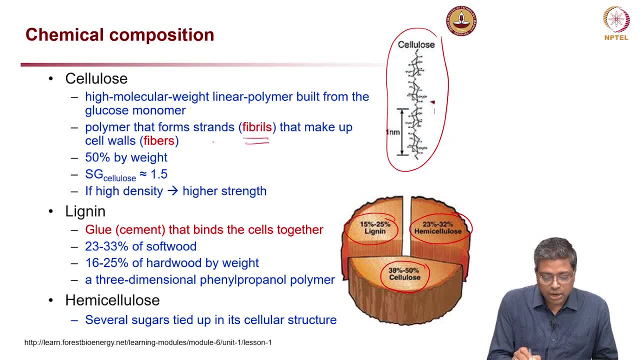 polymer that forms transfibril. Okay, These are fibrils that make up cell walls, fibers, These two things I will talk in the next slide. This fibrils and fibers. you will see in the next slide the same image I will show again. 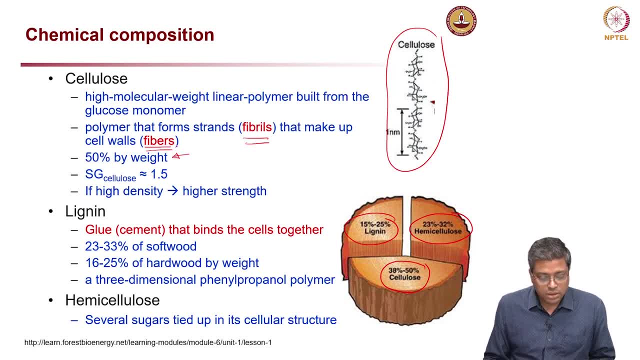 Now 50 percent by weight of wood is because of the presence of cellulose and its specific gravity is about 1.5. So in if high density and that leads to higher strength also, Okay. So lignin you know you have. it is basically the glue that binds the different cells together. 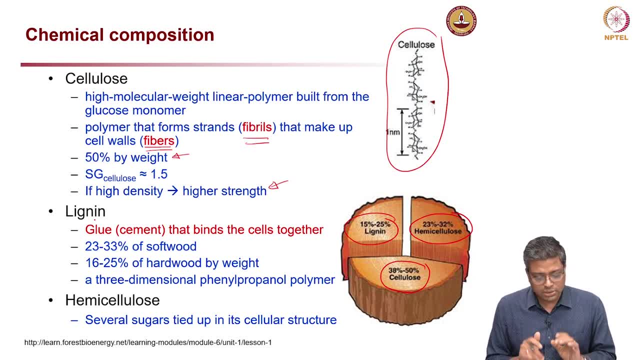 or the cementitious property. Essentially, it is a glue. Okay, That is what it is, and it is 23 to 33 percent of soft wood and, in case, if it is a hardwood, then it is. So these numbers, you know, I am not expecting you to memorize these numbers, because this 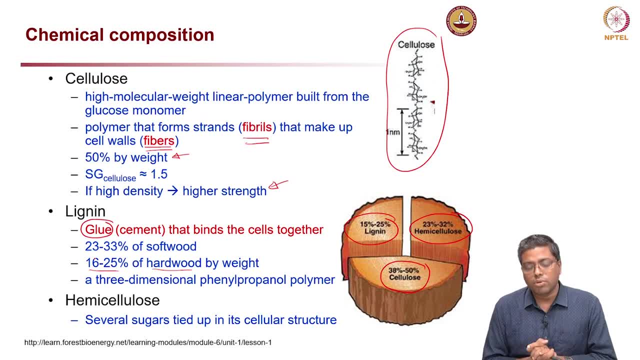 will vary from wood to wood. Okay, But just to have a ballpark idea About how much is the composition, etcetera, etcetera. Okay, Now what it is? lignin, a three-dimensional phenylpropanol polymer. Okay. 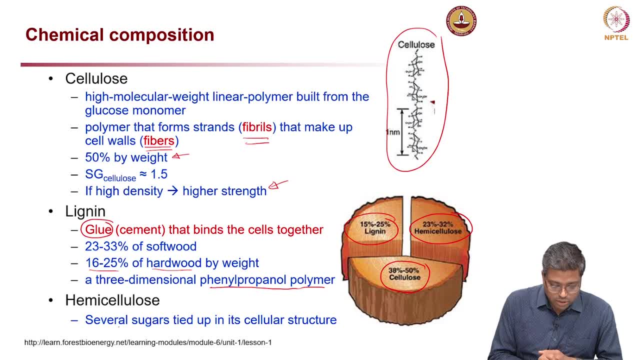 Anyway, so this general idea, only Now. hemicellulose, several sugars tied up in its cellular structure. So this is how the chemical composition main thing is to look at: which is the key component, which are the key components and what is a roughly the proportion and their role. 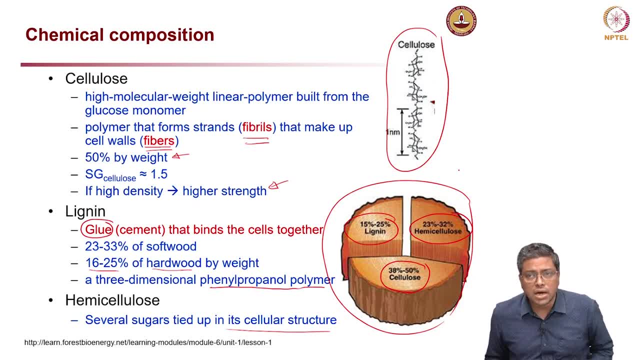 Okay, So all the most of the properties are, you know, provided by the cellulose, and lignin plays like a role of combining or binding these cells together and, you know, hemicellulose is where the different sugars tied up in a cellular structure. 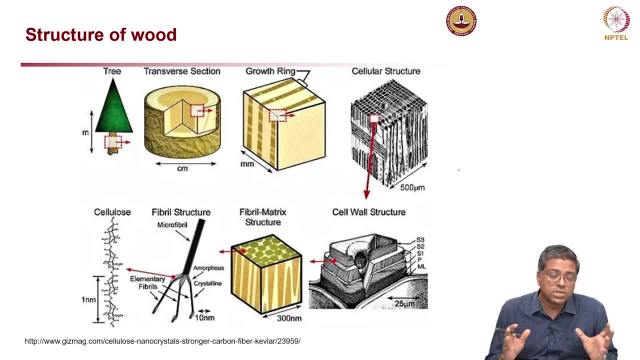 So this is what the chemical composition. Now look at the physical structure of wood. Physical structure: Okay, As we will start. from macro level to biodegradable, Okay, Okay, Micro level, That means from the top right, top left of the screen to the bottom right of the screen. 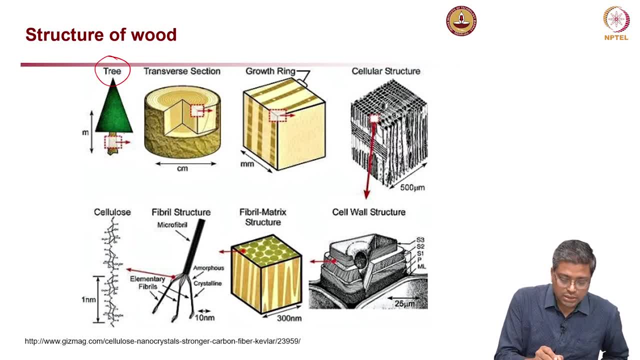 So let us see a tree. Okay, You cut a stem of a tree and that is this like this. If you cut it like that, what you will see, let us say, in the range of centimeters, Okay, A few centimeters. let us say, depending on what you are cutting, 10 centimeter or if it. 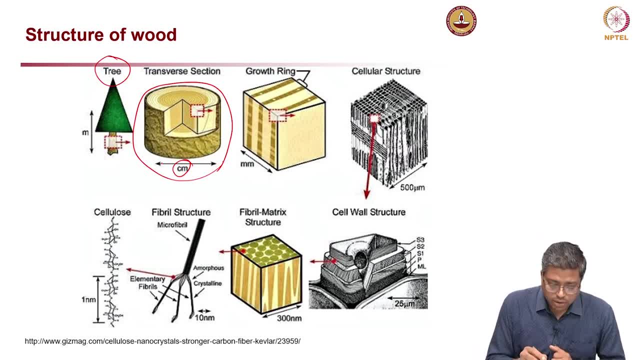 is a very large tree, might be even going into meters, Anyway, whatever that is. So you take a stem and then you can. you can look at these red squares or rectangles shown on each of these image here, which kind of indicate the next image which is zoomed in. 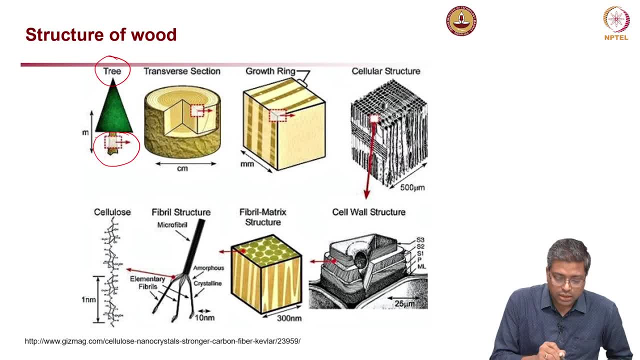 So from the first image I have a rectangle here, So the second image is the how that rectangle looks like the transverse section. Okay So, Now Another here. this is showing this thing, Okay. So, like that, zooming in, zooming in your, you know, sequentially getting more closer and 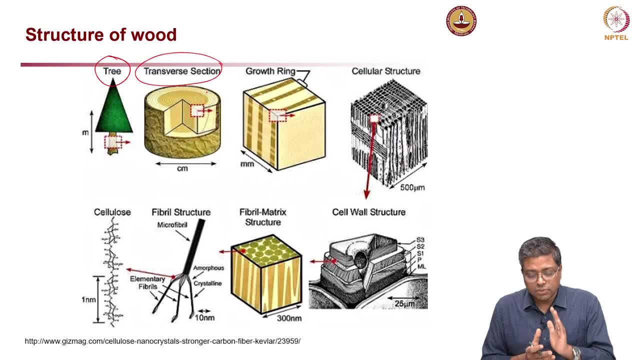 closer image. Okay Now, second, is very clear Now. third one: it is showing what are the rings which we talked about, the growth rings we talked about. very clearly you can see the growth rings, You can see the early wood and late wood here. 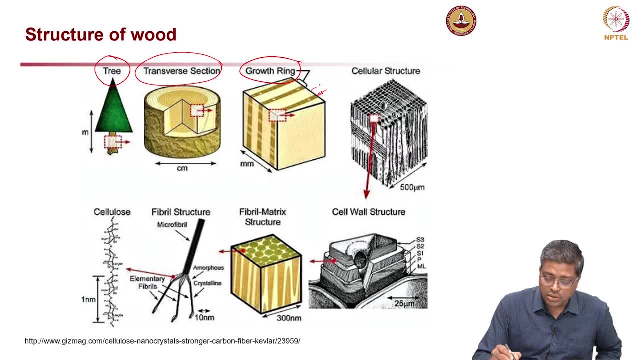 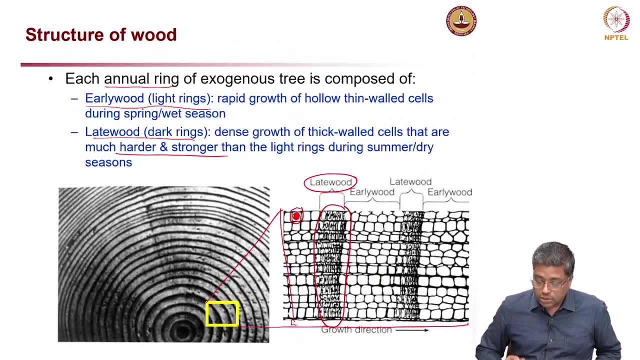 Right. So you can very clearly see this is the, this is the early wood and the late wood. So just to reemphasize that, So you can see here that denser one or the late wood and the lighter one or the early wood. 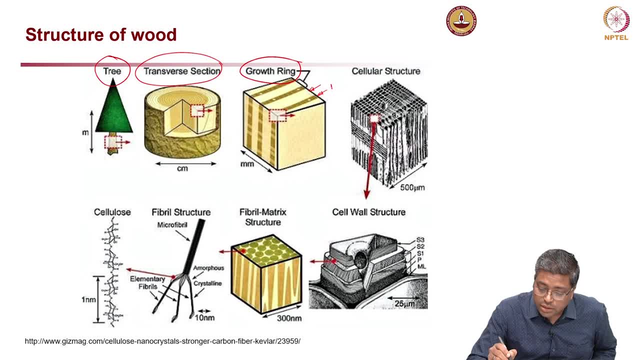 So so here you can see, this denser one is the early wood and the sorry denser one is the late wood And the lighter one is the early wood. Okay, So you can see, the denser one is the early wood and the lighter one is the early wood. 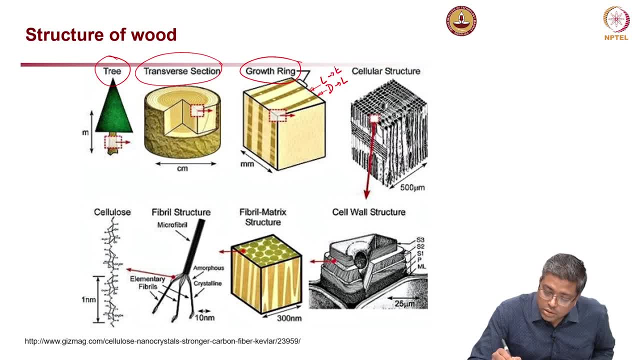 Okay, Anyway, Now, if you look at this region, here you can see the close up of that cellular structure, close up of the cellular structure. Now, here you can see, you have again these cell walls, These cell walls, etcetera, are visible here further going, 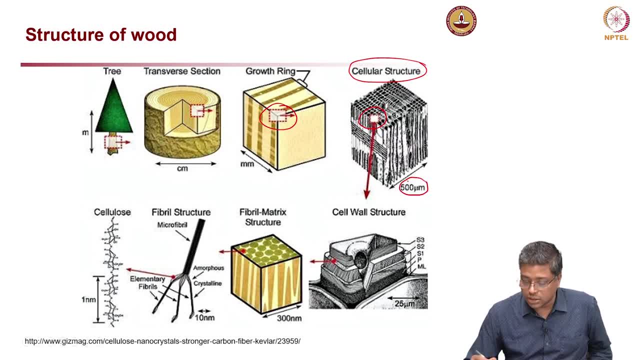 So you can also track the size in which you are talking. This is like about 0.5 millimeter, okay, So very small region. we are talking about this one. Now, if I go to the cell wall structure, I am sorry. I think I in the beginning I told that. 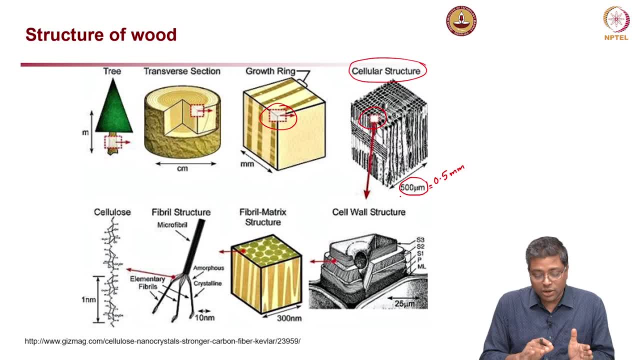 we will go from top left to bottom right. No, We are going clockwise direction, So going like this. and then we will go like this. okay, sorry So, top left to bottom left. that is how clockwise direction we are going. So here now you can look at the cell wall structure, where you can see different again. 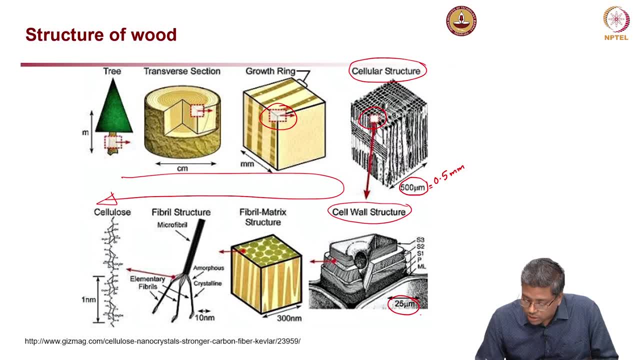 microstructure level, you can see 25 micrometer. that means 0.025 millimeter, So you can see how small we are looking at. Okay, And then looking at one of the cell wall element. okay, So here that is. this is how the cell wall element looks like. fibril matrix, how the fibrils. 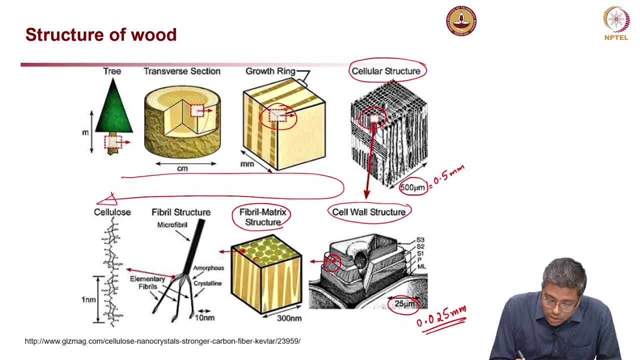 looks like. and then you can see here: these are all each of those fibrils. okay, All these green circles here are individual fibrils. Now, next image on the left side, looking at fibril. Okay, Fibril structure. you can see microfibrils and amorphous structure, crystalline structure. 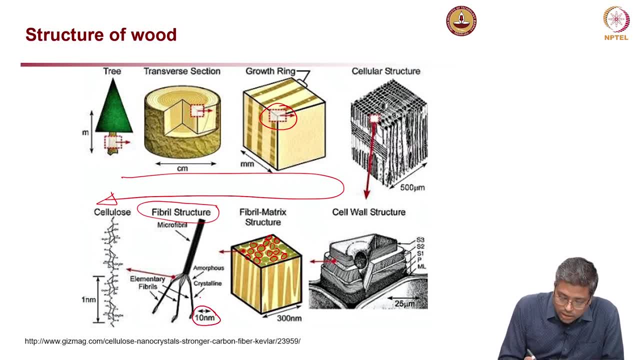 depending on what type of tree it is, and then you can see it is also very, very small, 0.01 millimeter. sorry, this is nanometer, right? So it is sorry it is. you can see it is nanometer, very small nanometer, Okay. 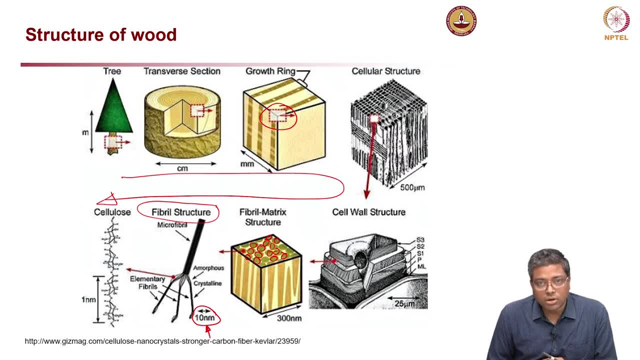 Okay, So 10 nanometer scale, you are talking about that. Then further, if you go into the chemical structure, you can see cellulose. this picture I already showed in the previous slide. okay, So this is in general the physical structure of wood. okay. 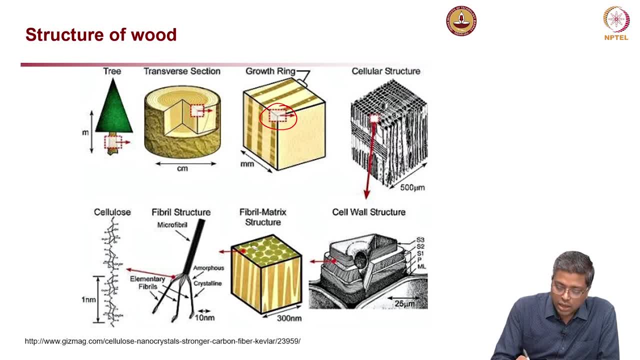 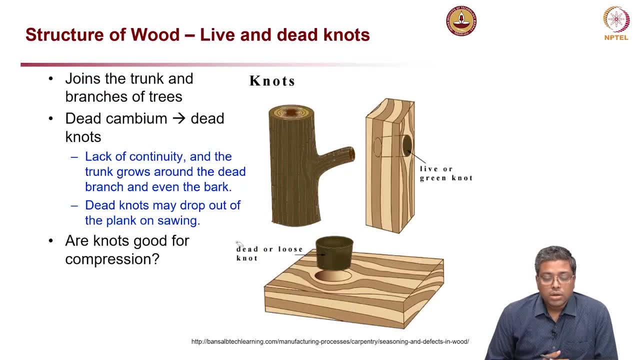 So you can start from how a tree looks like and all the way into these small chemical structure of the wood. Now, Okay, So if you look at the physical structure, there are something which you might have already seen on wood. there are something called knots. okay, 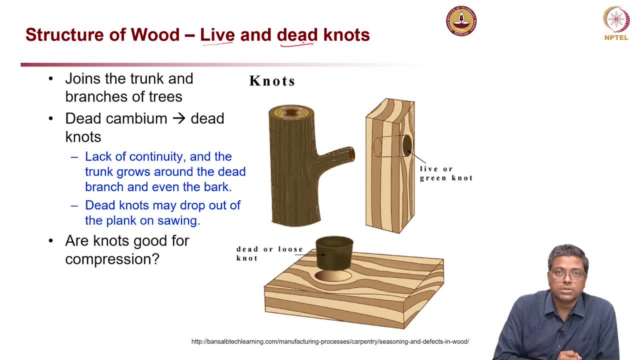 And also there are live knots and dead knots. How do they function? or what is the role? you know, how do they influence the properties of the wood? So what they are essentially is they join the trunk and branch of a tree. So if we can think here, 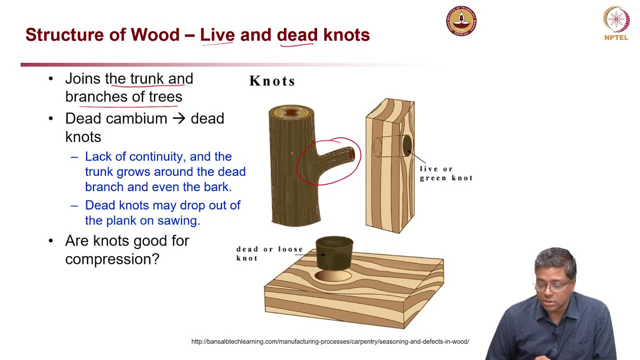 This is where a branch is coming out of a trunk, Okay, Or a stem. And now if it is live or green knot, it will be something like this: Okay, that means it is active, they are connected together, they are bonded well together. Now, if it is a dead knot, like this shown on the bottom right image, okay. 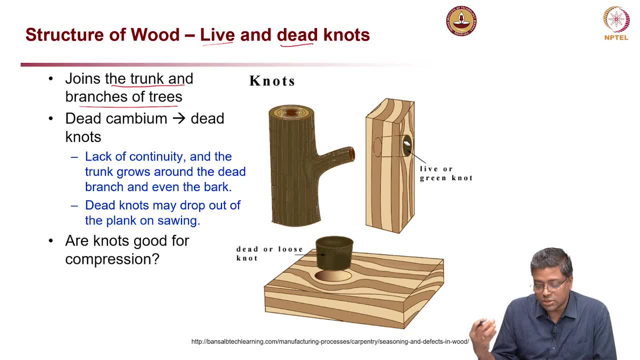 You can see that it is not really mechanically. it is not bonded to the wood. So if you just try to pull it out, it will come off okay. Now this has a problem, or wood or timber with this kind of knots may not always be good. 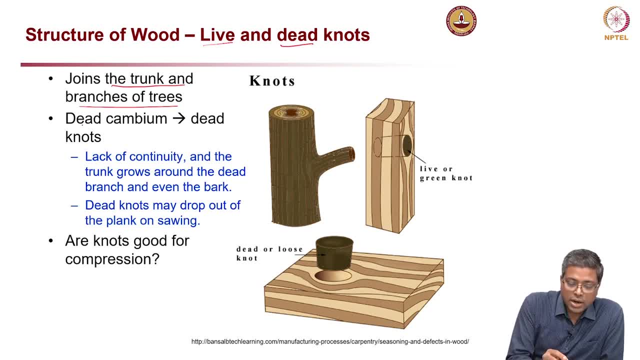 when you look at mechanical behavior. So what happens is why this is happening- is the cadmium, which is the growing part of the wood. like you know, I said no thin layer between the bark and the, the growing between the bark and the hardwood, or Okay? 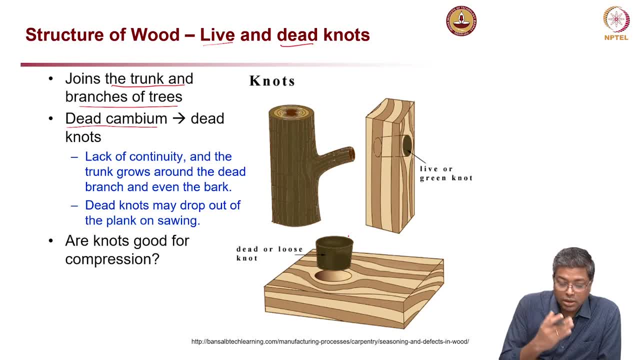 The sapwood, between the, between the sapwood and the bark, So this thin layer of cadmium that actually, if that gets dead, then the knots also get dead because there is no further connection between them. So now, because of that, there is a lack of continuity. 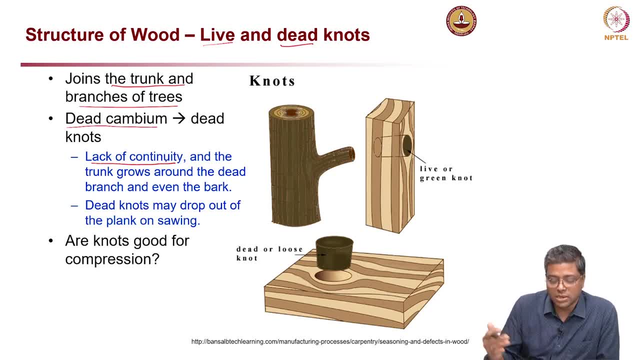 So it also affects the. you know the stress transfer, etcetera, And the trunk grows around the dead dead branch and even the bark. The dead knots may drop out of the plank on sowing, but there are also cases where you might have it inside the wood but it is not just falling off, but it stays there. 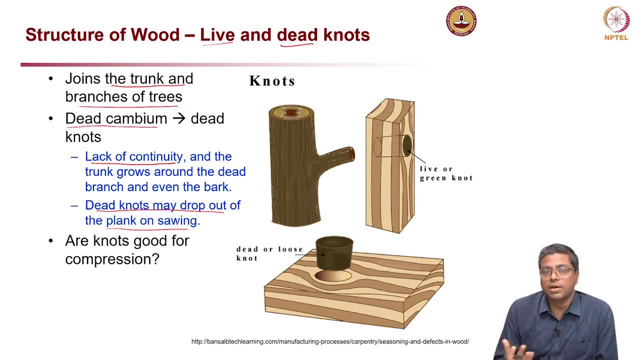 But the way you apply the loading, it might have an influence on the behavior. okay, So the question here is: are knots good for compression? Now look at this picture here: Okay, If I compress this wood like this. okay, and like this, if I compress the wood like in the 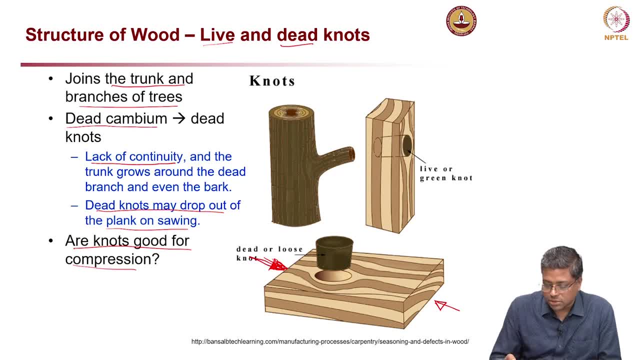 direction parallel to the grains. if I compress, if I compress the wood in the direction parallel to the grains, okay, what will happen is there will be a lateral force generated here, lateral stress will generate here and it like this- Okay, And it can this- the stress concentration will happen here and here and it can actually lead. 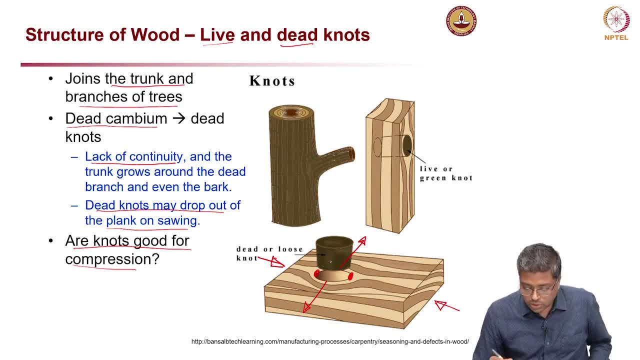 to failure of the wood because of the dead knot there, And also it will. it might push out, also push out the dead knot. that is one thing. Now if I apply a load in the other direction, let us say I am applying the load in this. 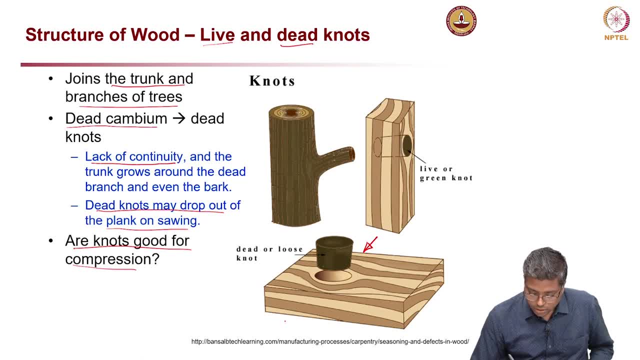 direction: Okay, Okay, Okay. Then also there is a compression and it might push the knot out, but again you might experience that there is a stress concentration but depending on the direction it might not affect much in this direction, but in the other direction which I showed you earlier, it will definitely. 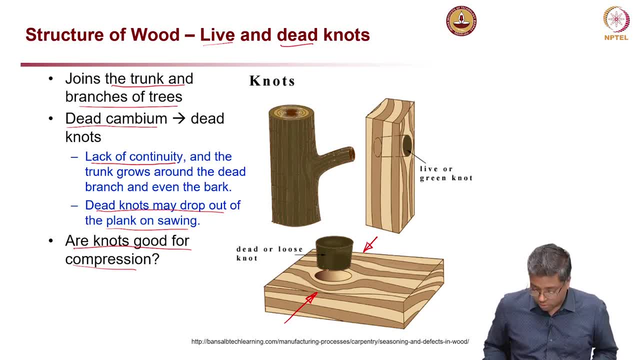 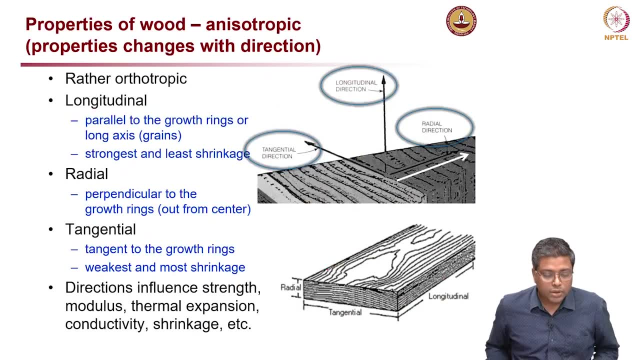 have some impact on opening up or, you know, cracking of the wood along the grains or between between the grains. Now, properties of wood: they are anisotropic in nature. that means they are very much dependent on the direction. okay, So I would say even rather orthotropic in nature, but again, let us say it is anisotropic. 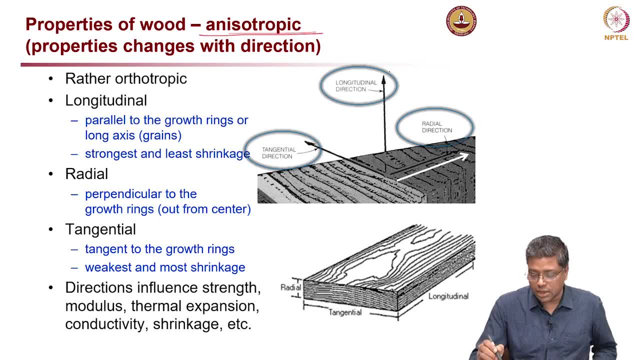 is the key word which we are talking here Now, in the longitudinal direction, that is, this direction, in that is, along the stem or along the grains, Parallel to the growth rings, parallel to the axis of the growth rings. okay, Now they are strong in that direction and least shrinkage happens in that direction. 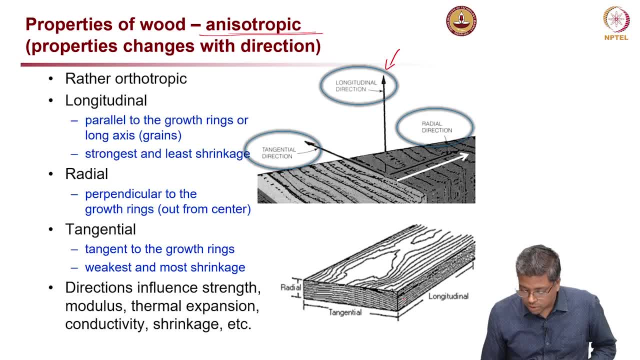 okay, So that means the look at the picture on the bottom right. you can see this is the longitudinal direction I am talking and these are all the grains. you can see on this and along the grains they do not shrink much, okay, Okay, So shrinkage in this direction is very minimal. shrinkage in this direction is very minimal. 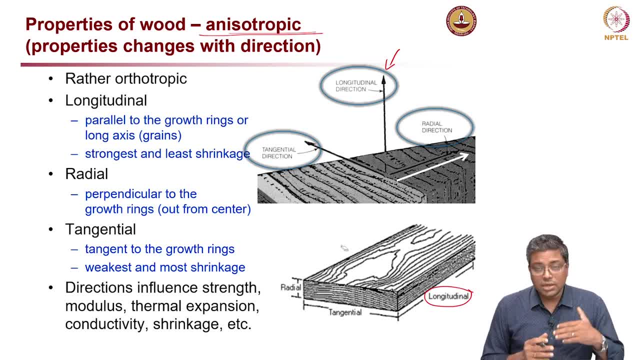 Now, if you look at the perpendicular direction- either radial or tangential direction- okay, Either radial or tangential direction, you will have you know the weakest or weak. the strength is weak in that direction And shrinkage happen mostly in these directions. okay, Shrinkage happens, so this will shrink this way or it will shrink this way. this is what. 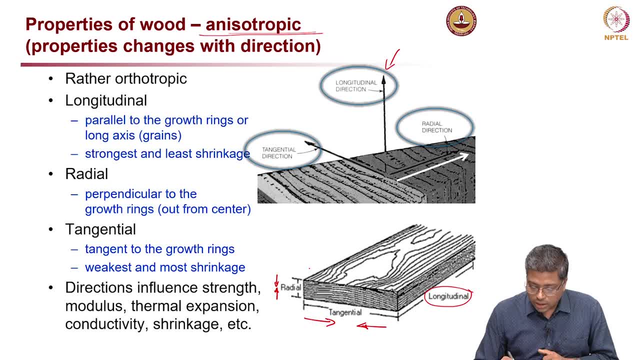 we are talking about, But the shrinkage in the longitudinal. this shrinkage is very less okay. Here it is more, here also it is more okay. So I think that is clear. So directions influence the strength, The modulus, the thermal expansion, conductivity, shrinkage, all these mechanical properties are 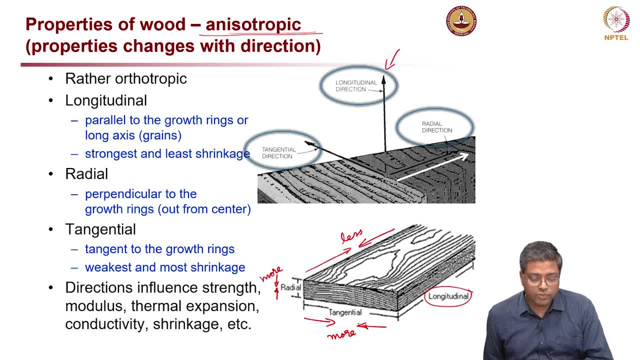 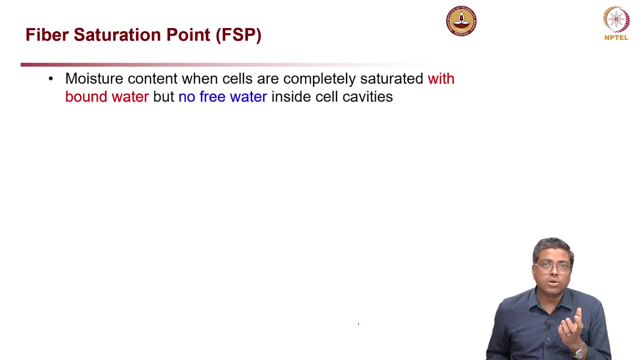 very much different in these three directions of a timber, okay, Especially between the longitudinal and the other two directions. Now there is something called fiber saturation point. What is that? So this is the moisture content when cells are completely saturated with moisture. This is the moisture content when cells are completely saturated with water. 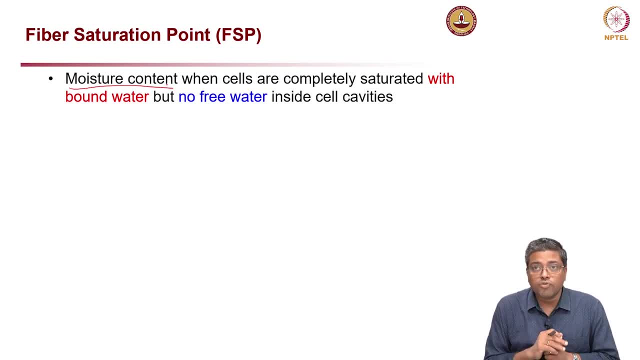 The water which is chemically bound, and but no free water inside the cavities, inside the cell cavity. So the cell walls. okay, The cell wall. let us say this is the cell wall. okay, So the cell walls here. let me draw it again. 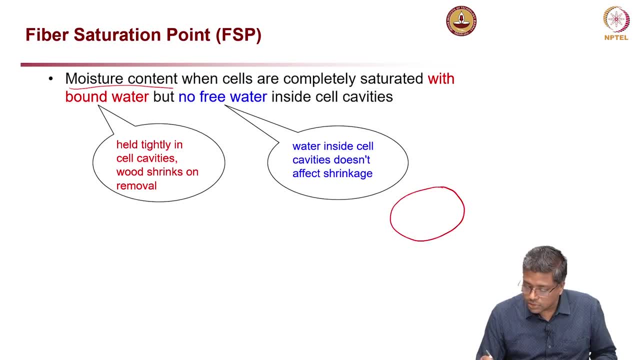 So it says cell cavities. Assume that this is a. this is a cell wall. Okay. So it says Cell cavities, cell, wood, cell and these are the. this is the cell wall. okay. Now, the highly you know. 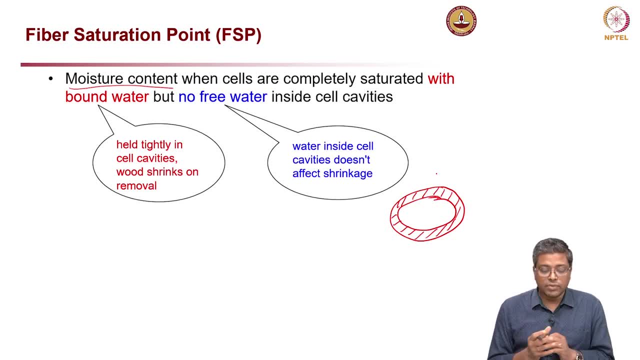 the water is held tightly in cell cavities, wood shrinks and removes. So this is the bound water which you are talking and the water inside the cavity. the second one is this one: the water inside the cavities does not affect the shrinkage. okay, So first, when you try to dry wood, 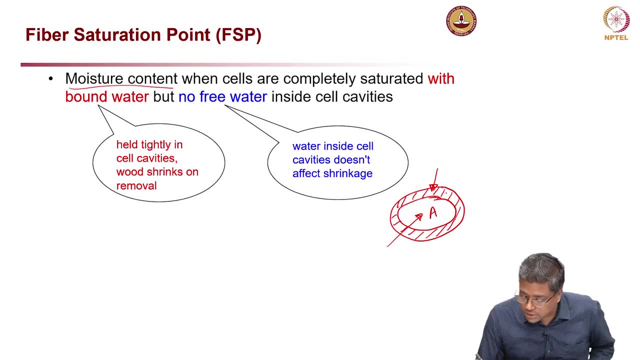 what will happen is first, let us say I am going to call this region A and then region B. okay, First what will happen is the water in the region A will evaporate, that is the free water, and then, after further drying, then only the water. 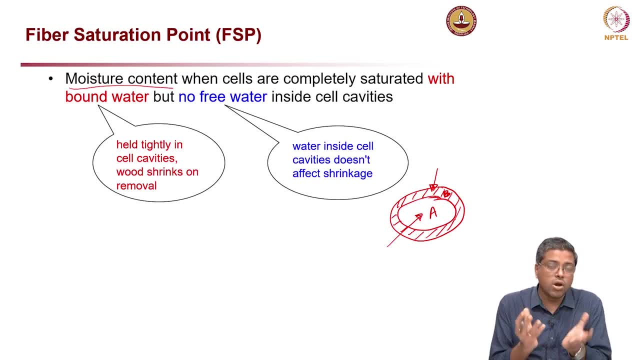 in the region B, or that is, the cell wall itself will start evaporating. okay, Now FSP is about 20 to 30 percent for most of the wood. So above the FSP that means if the water you know, 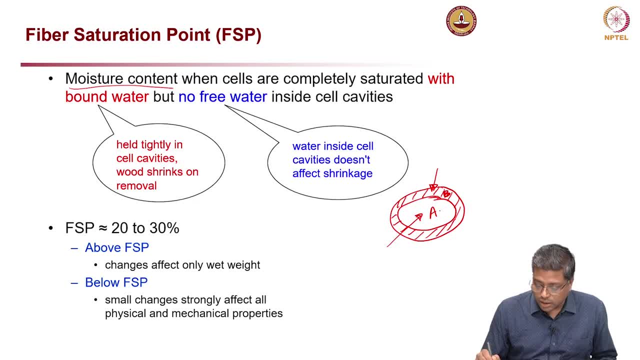 content. if there are still water in the region A, okay, then it affects only the weight and below FSP. what happens, is it? it below FSP means you are now start taking the water from the region B and then the properties start getting affected, like physical and mechanical properties will start. 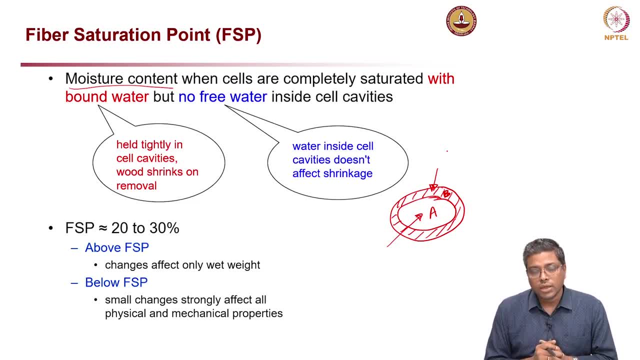 getting affected. Let me reiterate this once more. Let us say you: you take a new wood, you cut it, you are going to process it and now you have to first dry that wood right? So initially you will have a lot of moisture in the wood. Now, as you start, 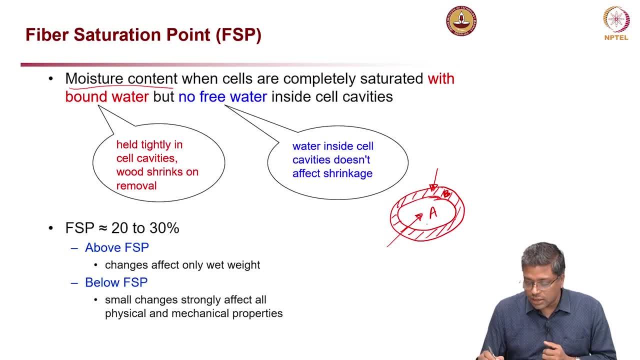 drying first the water in the inside the cell cavities, that is the region A, will start drying. okay, At that time the only change in the wood is the change in the weight of the wood, loss of water. Now, after further drying, when you reach like fiber saturation point at that time then 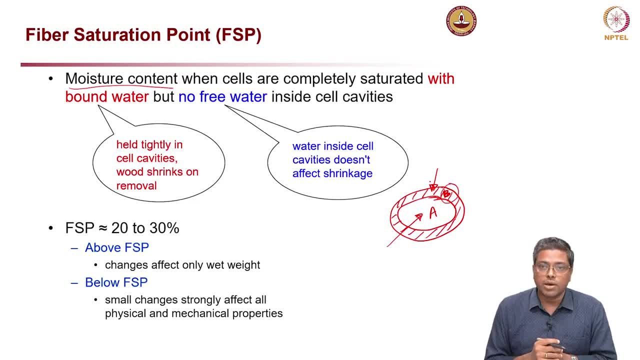 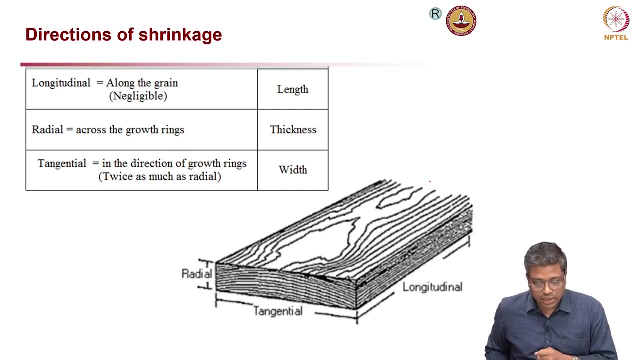 the water from the region B also start evaporating and then the properties start changing, not only weight, but also the shrinkage and mechanical properties starting- And now I am going to show you this thing once more. This, this sketch, is just to. 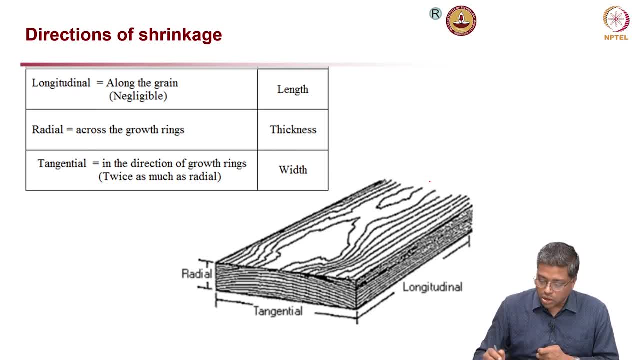 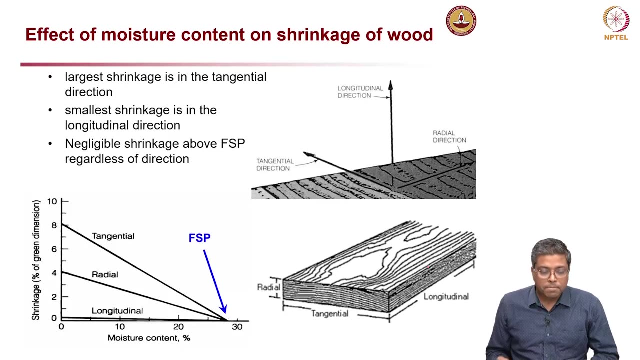 tell you about the direction of shrinkage in the longitudinal direction. We have already discussed this. in the longitudinal direction it is negligible, you know, and in the tangent radial and radial direction there is a twice as much difference in general. Now, this is what we were just talking about. what is FSP? 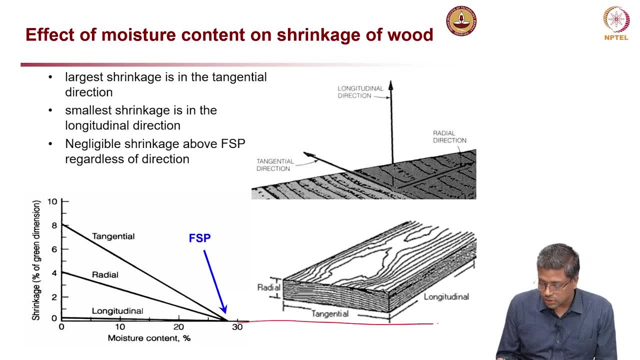 So let us say- I am extending this, this to the right. Let us say: this is about 100 percent okay, Fully saturated wood now? okay, Now what happens? you start. you have to go for from the right end of the graph to the left. so this is how we start drying the wood. 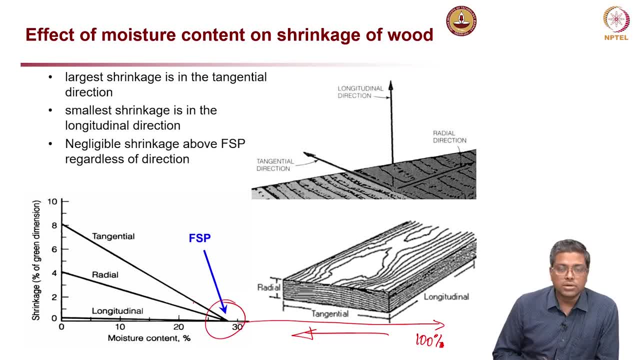 So up to about 20 to 30 percent. that is this region. here there is no change in the shrinkage property because the water from the cell cavity is being evaporated. So this is what I drawn earlier. this is B region and this is A region. 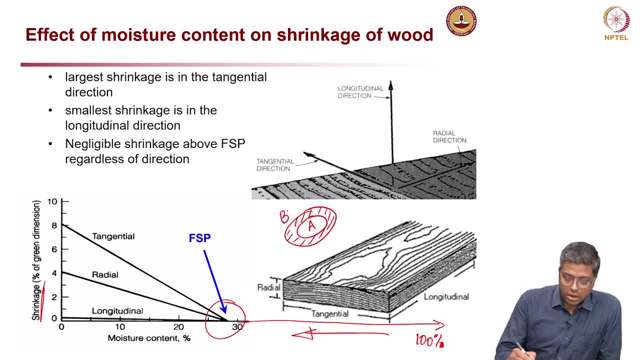 So from water, from the cell cavity is evaporated. so after this 20 to 30 percentage you can further drying. you are removing water from the wall region, that is the B region, and that leads to change in the properties. So largest shrinkage happens in the tangential direction and then smallest shrinkage in the